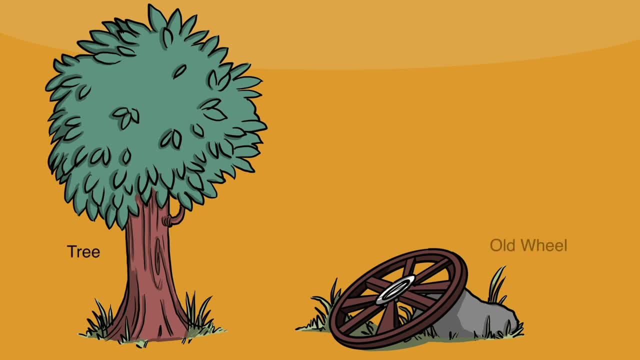 side we have a tree, and on the right side we have an old wheel that has been dug up out of the ground. Now we know that all living things are made of carbon, and a certain percentage of that carbon is always carbon-14, which is radioactive. So let's look at the count. 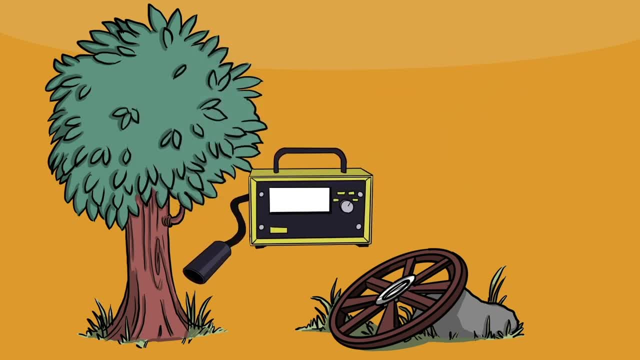 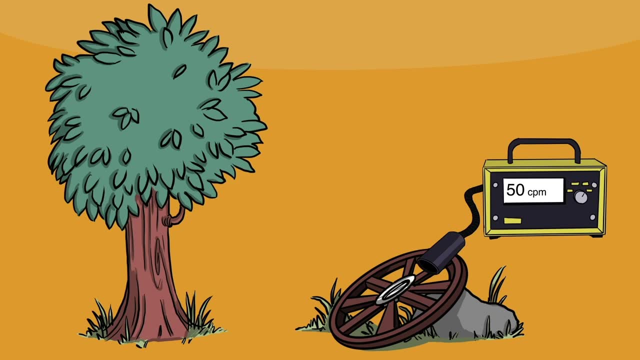 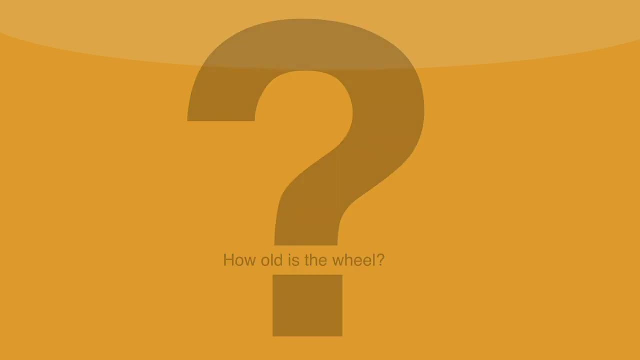 rate of a tree that's still alive. We see that it's 200 counts per minute. Now let's look at the cartwheel. The count rate here is only 50 counts per minute. So how long is it since the wheel was made? How old is the wheel? First we need to find out how old 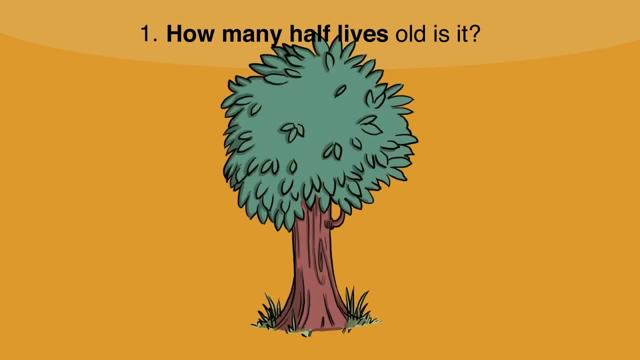 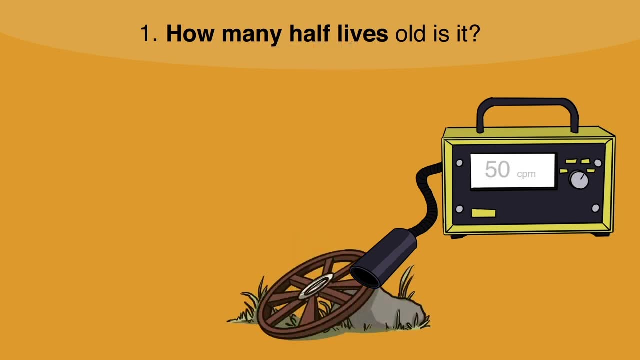 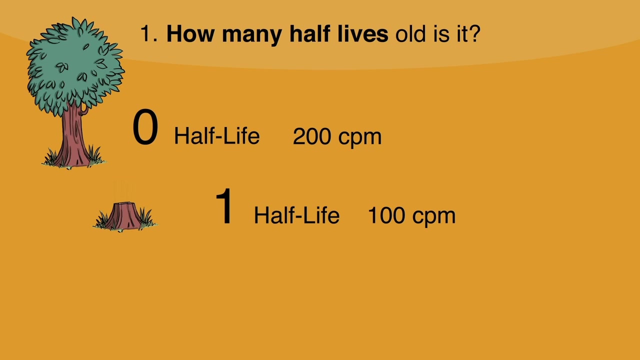 how many half-lives old it is. With the count rate of a tree that's alive is 200. And when that tree is cut down and turned into a wheel, that activity will slowly start to reduce. Then after one half-life it would reduce to 100, and then after two half-lives it would 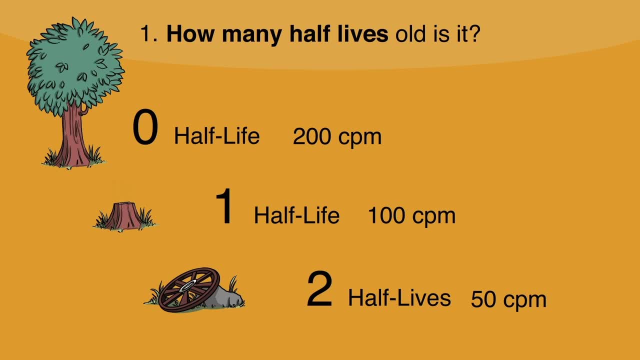 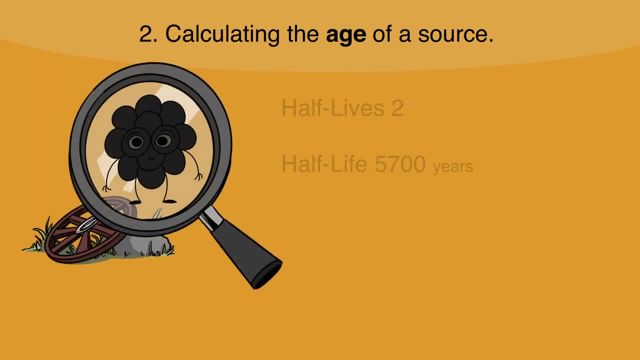 reduce down to 50, which is exactly the count rate of the wheel. So we know that that wheel must be two half-lives old. Now we know that the half-life of carbon-14 is 5,700 years. So if it's two half-lives old, it must be two times 5,700,. 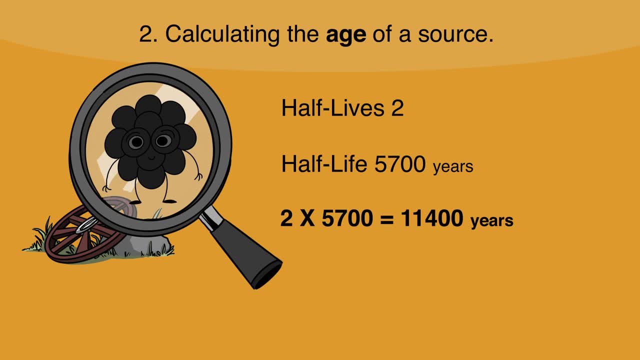 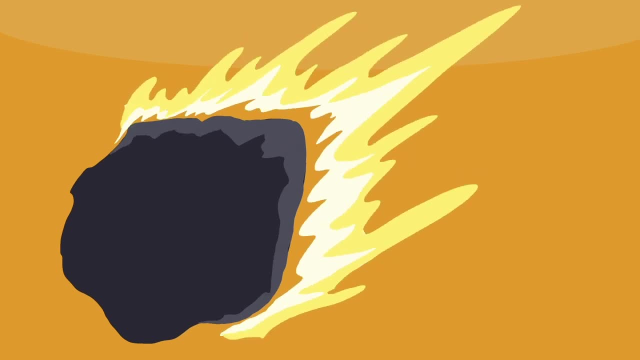 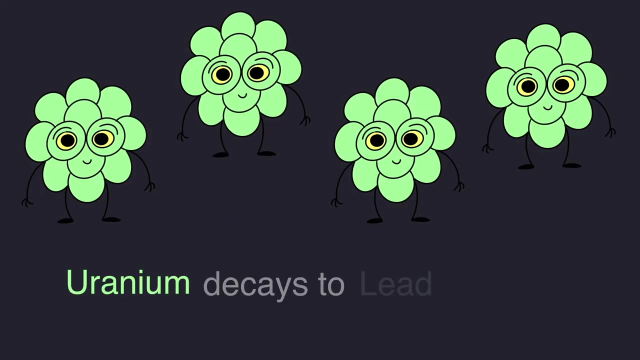 which is 11,400 years old, And that's it. That is radioactive dating. Let's look at another example. So here we have a meteor that's crashed to Earth, And we know that when the meteor was created, it was all uranium, But uranium decays to lead And now there's only one uranium atom. 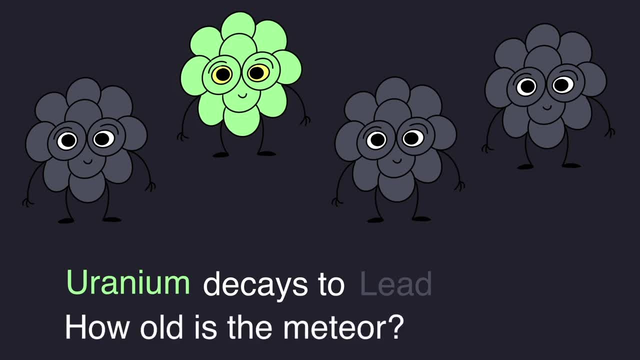 to every three lead atoms. So how old is the rock? Well, first we need to find out how many half-lives old the rock is. There's one uranium atom to every three lead atoms. So a quarter of the rock is uranium. How many half-lives would it take to get to a quarter? Well, if we start at one, 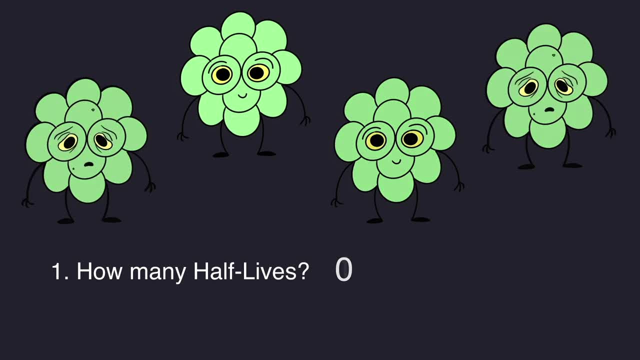 when all the atoms are uranium, then after one half-life it's only a quarter. So how many half-lives would it take to get to a quarter half-life? half of the atoms would be left as uranium And then after two half-lives,